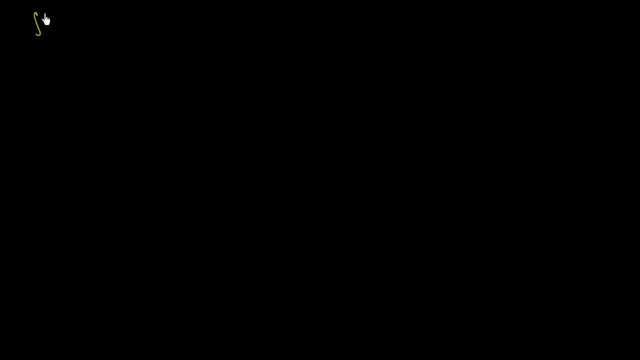 Let's now prove the divergence theorem, which tells us that the flux across a surface of a vector field- and our vector field we're going to think about- is f, So the flux across that surface, and I could call it f dot n. 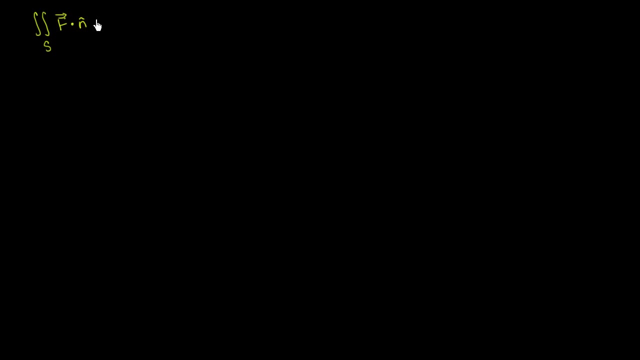 where n is the normal vector of the surface and I can multiply that times ds. So this is equal to the triple integral summing up throughout the volume of that region, summing up that volume of the divergence of f. And we've done several videos explaining the intuition here. 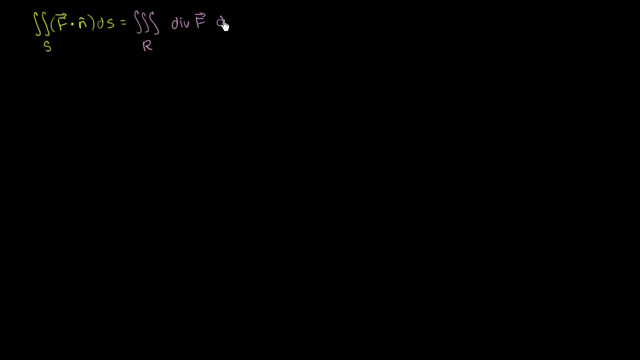 but now we are actually going to prove it And of course we're times each little differential cube of volume And we're going to make an assumption here. We're going to assume that we're dealing with a simple, solid region And what this means more formally. 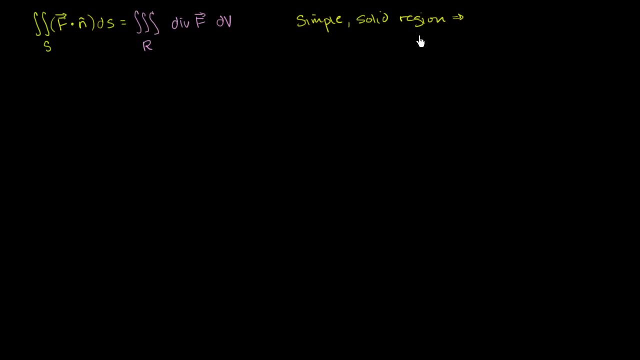 is that the region we're thinking about can be a type 1,, type 2, and type 3 region, Or I should say it is all of the three, So it is types 1,, 2, and 3.. 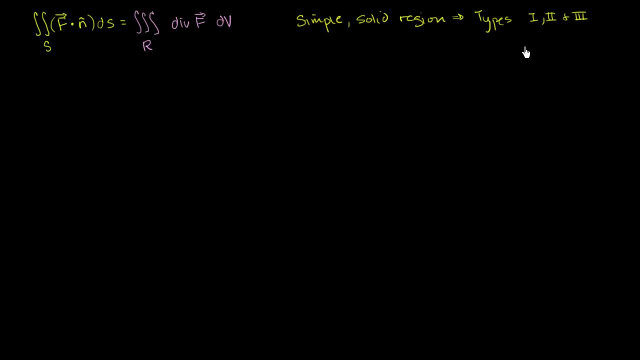 And there are videos that go into what each of these regions are, but a lot of the basic shapes fall into this simple, solid region, like a sphere or a cylinder of some kind. They can be types 1,, type 2, and type 3.. So they're not the same region. They're not the same thing, So they're not the same thing. They're not the same thing, So they're not the same thing. So they're not the same thing. So they're not the same thing. 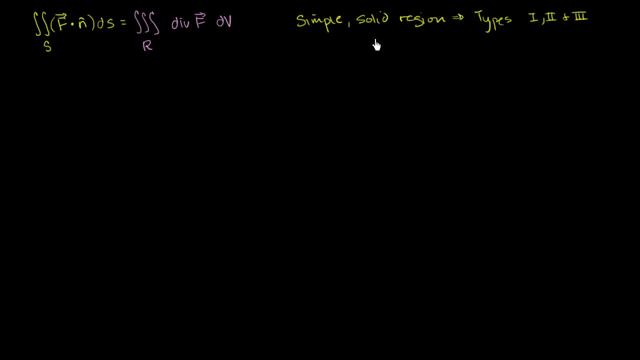 And for a lot of situations that aren't simple solid regions. you can break them up into simple solid regions, But let's just prove it for this case right over here. So let's just assume that our vector field F can be written as p, which is a function of x, y and z. 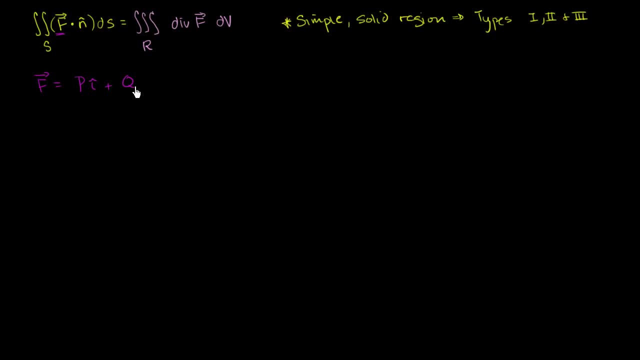 times i plus q, which is a function of x, y and z times j plus r, which is a function of x, y and z times k. So let's think about what each of these sides of the equation would come out to be. 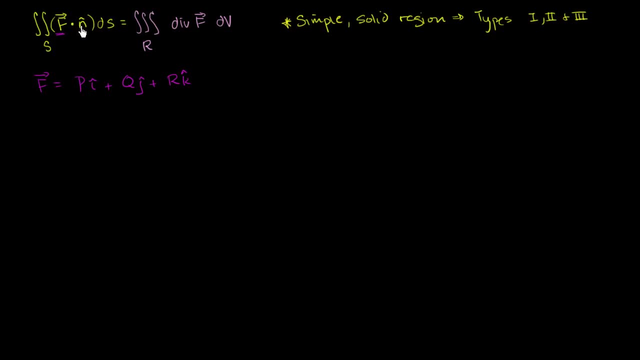 Well, first of all, what is going to be F dot n? So let's think about that a little bit. F dot n is going to be equal to this component right over here, times n, So n's i component, plus this component right over here, times n's j component. 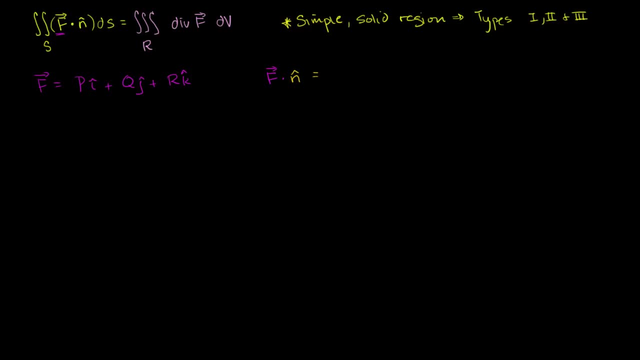 plus this component here, times n's k component, So we could write it as it could be written as p times, or I'll just write p, open parentheses. the dot product of i and n. i dotted n and let me make sure I write i as a vector, as a unit vector. 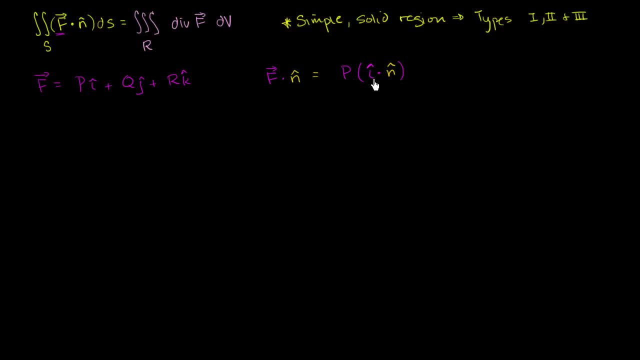 And what I'm going to do. I want to be clear What's going to happen right over here. If you take the dot product of i and n, you're just going to get the i component, the scaling factor of the i component of the n normal vector. 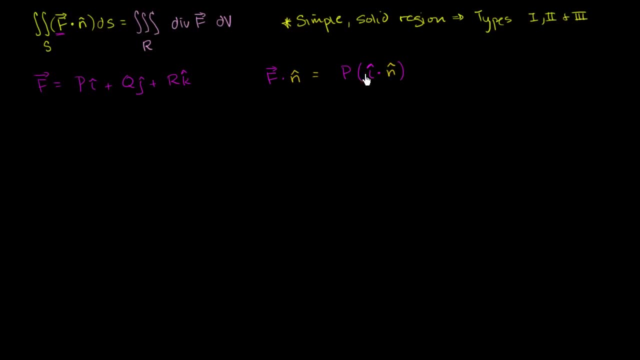 and we're just going to multiply that times p. So that's essentially the product of the x components, or I guess you could say the magnitude of the x components, And then to that we are going to add q times j. j dotted with n. 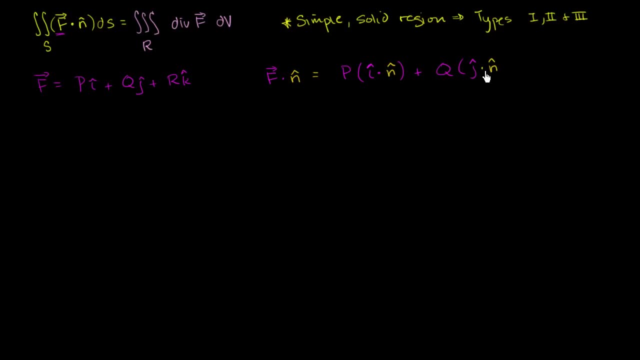 And once again, when you dot j with n, you get the magnitude of the j component of the normal vector right over there, And then times, or plus, I should say plus r, times k dotted with n. This isn't how we normally see it. 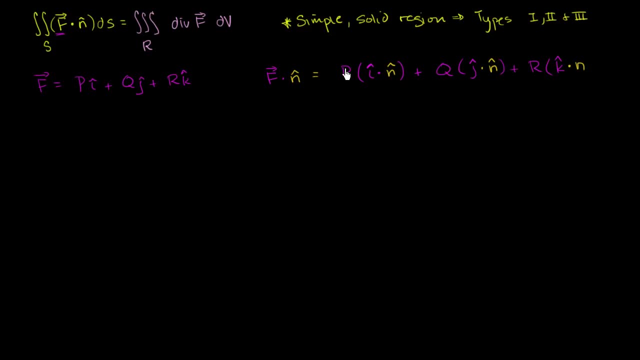 but I think it's reasonable to say that this is actually true. This right over here is going to be equal to p times the magnitude of the i component of n's normal vector, which is exactly what we want in a dot product. This is the same thing for the j component. 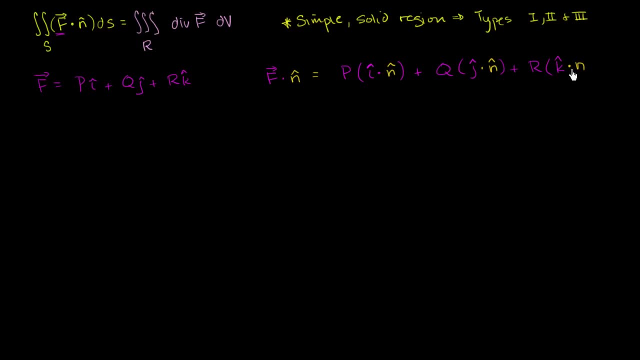 This is the same thing for the k component, And you could try it out: Define n as equal to I don't know m times i plus n times j plus o times k, or something like that, and you'll see that this actually does work out fine. 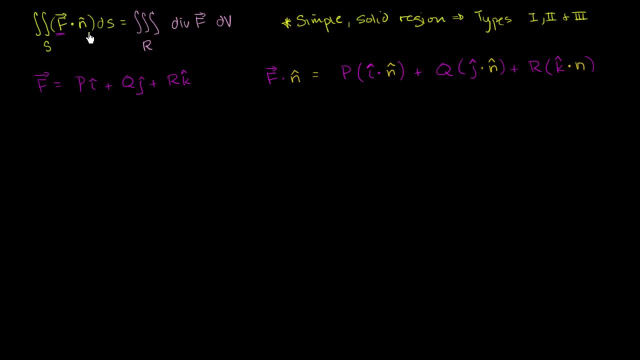 So how can we simplify this expression right up here? Well, we can rewrite this as we can rewrite the left-hand side as so: the surface integral of f. now let me write it multiple ways: f dot ds, which is equal to the surface integral of f dot n. 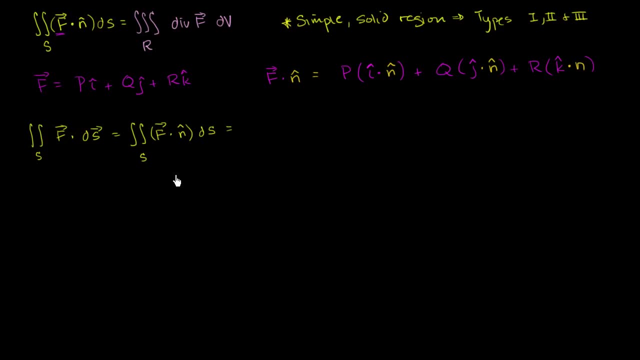 times the scalar ds is equal to the double integral of the surface of all of this business right over here is equal to the double integral over the surface of. let me just copy and paste that of all of that business. So let me copy and then let me paste. 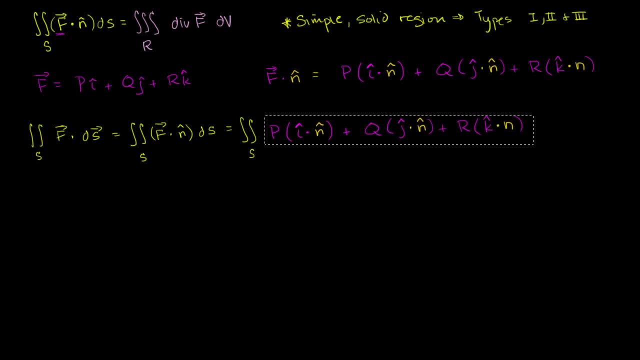 So all of that business right over there. I just noticed that I forgot to put the little unit vector symbol, the little caret, right over there. put some parentheses, put some parentheses, and then we are left with our ds. And then this: 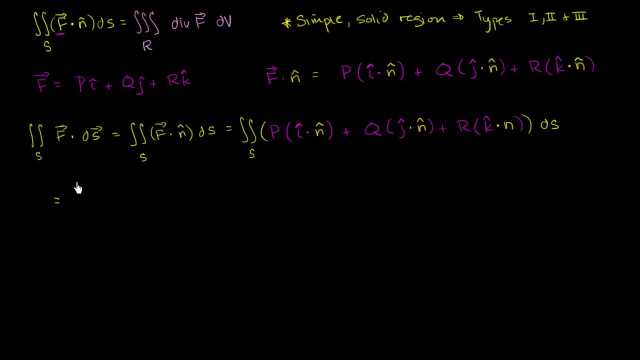 all of this can be rewritten, as this can be rewritten as the surface integral of p times this business, and I'll just do it in the same color of p times the dot product of i and n ds plus the surface integral of q. 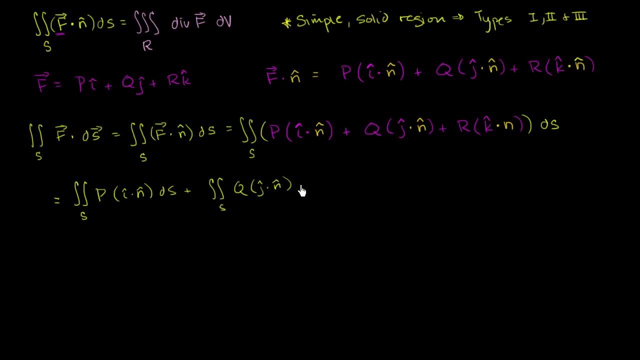 times the dot product of j and n? ds, plus the surface integral of r times the dot product of k and n. I forgot the caret k and n? ds, So I just broke it up. We were taking the integral of this sum. 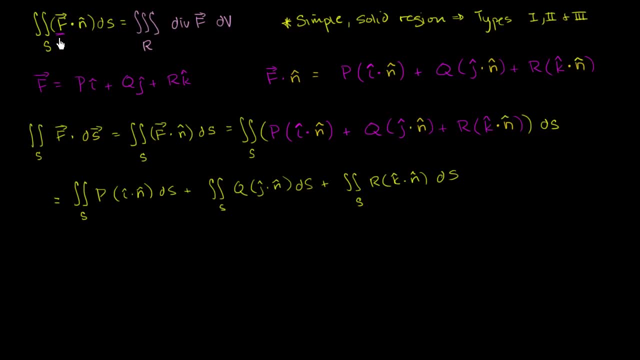 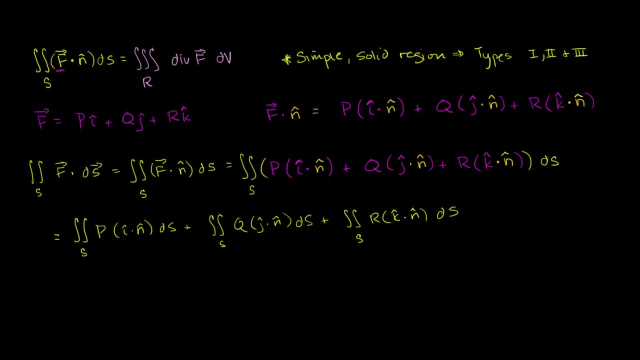 and so I just took it, as I just rewrote it, as the sum of the integrals. So that's the left hand side right over here. Now let's think about the right hand side. What is the divergence of f? And actually I'm going to take some space up here. 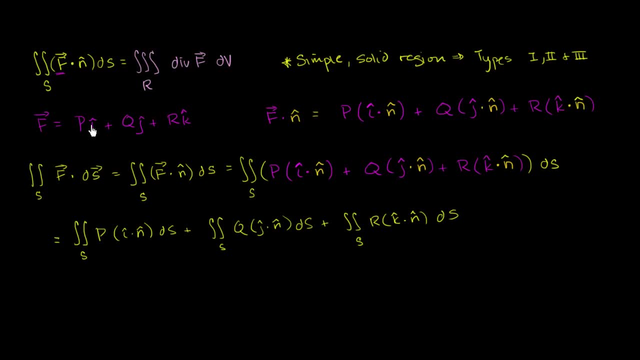 What is the divergence of f? Well, the divergence of f based on this expression of f is just going to be- let me just write it over here- real small. the divergence of f is going to be the partial of p with respect to. let me do this in a new color. 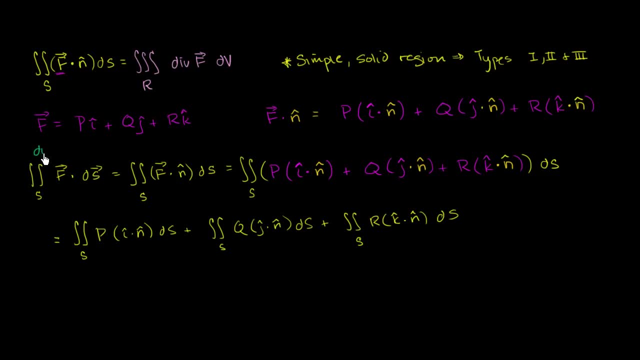 just because I'm using that yellow too much. The divergence of f. the divergence of f is going to be the partial of p with respect to x, plus the partial of q with respect to y, plus the partial of r, plus the partial of r with respect to z. 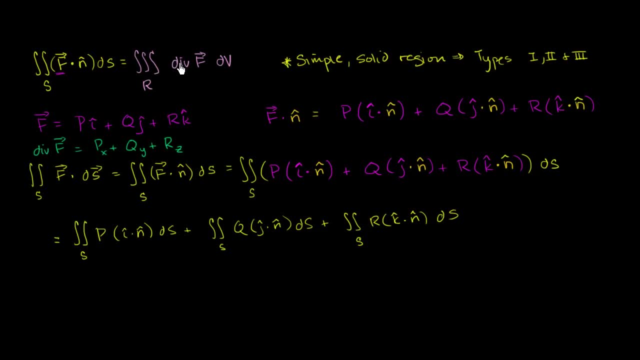 So we can, this second or this triple integral right over here could be written as the triple integral of the partial of p with respect to x, plus the partial of q with respect to y, plus the partial of r with respect to z. 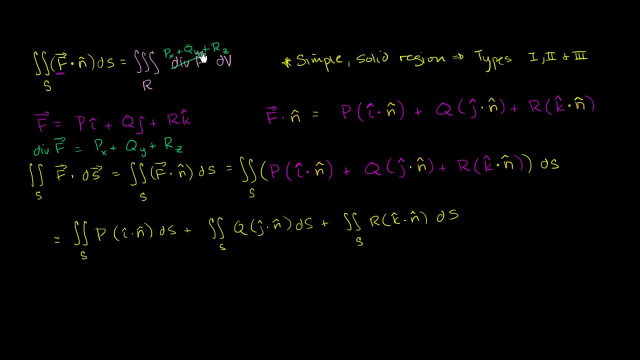 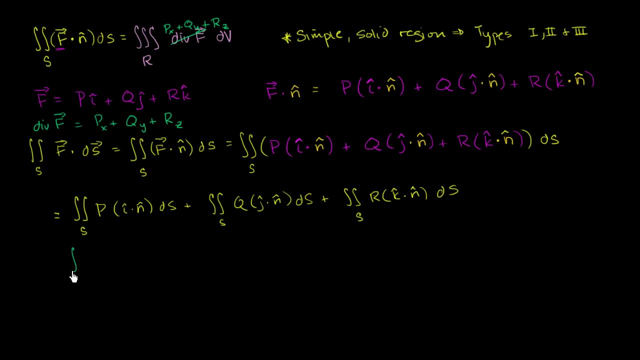 Well, this thing once again, instead of writing it as the triple integral of this sum, we could write it as the sum of triple integrals. So this thing right over here could be rewritten as the triple integral. triple integral over our three-dimensional region. 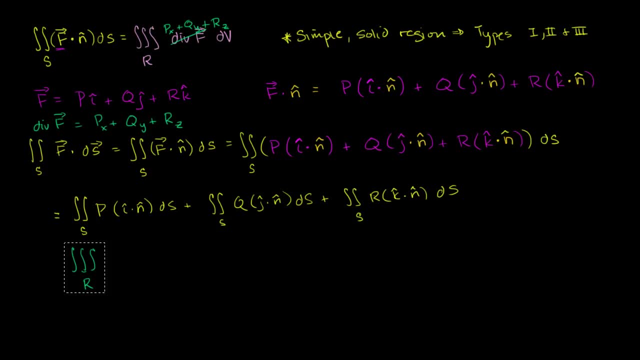 Actually, let me copy and paste that so I don't have to keep rewriting it. So let me copy it. So it's going to be equal to the triple integral of the partial of p with respect to x, dv plus. let me paste that again. 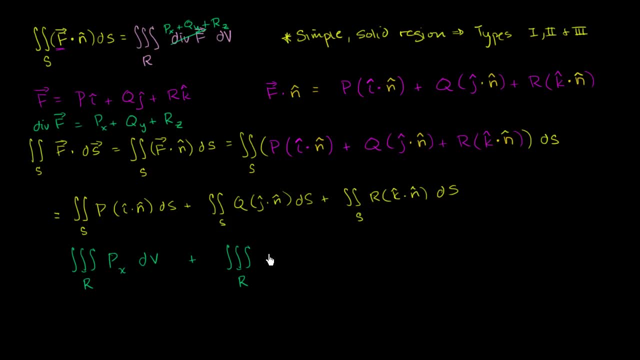 the triple integral of the partial of q with respect to y dv, plus, once again, triple integral, triple integral of the partial of r with respect to z, partial of r with respect to z dv. So we've essentially restated our divergence theorem. 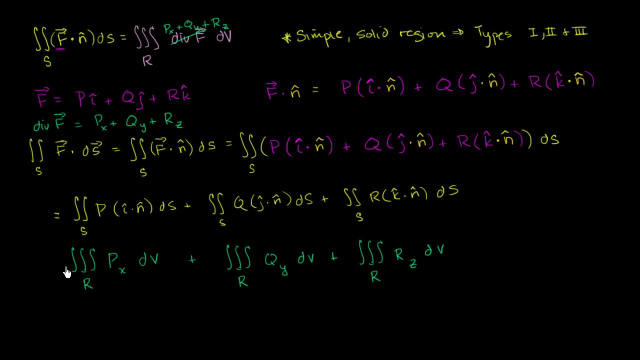 This is our surface integral, and the divergence theorem says that this needs to be equal to this business right over here. We've just written it in a different way, And so what I'm going to do in order to prove it is just show that each of these corresponding terms: 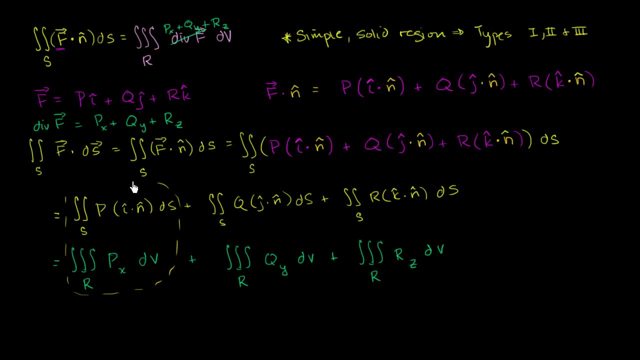 are equal to each other, that these are equal to each other, that these are equal to each other and that these are equal to each other And, in particular, we're going to focus the proof on this and we're going to use the fact. 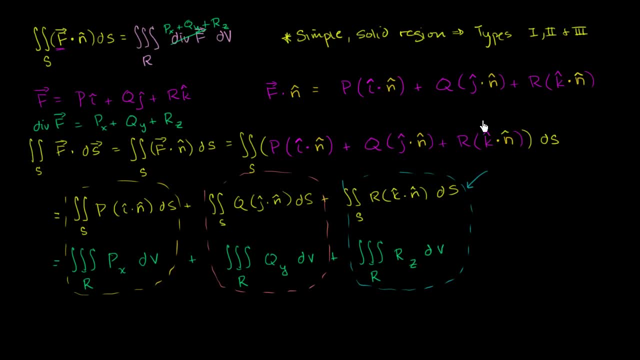 that our region is a type I region. It's a type I, type II and type III, But we're going to use it, the fact that it's a type I region, to prove that these two things are equivalent, And then you can use the fact that it's also. 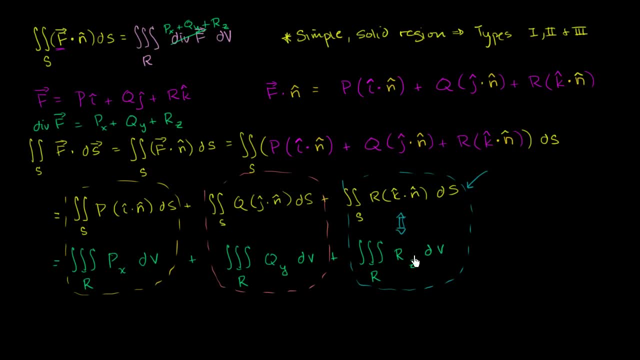 a type II and type III region, to make the exact same argument as to why this is equal to this and why this is equal to that.